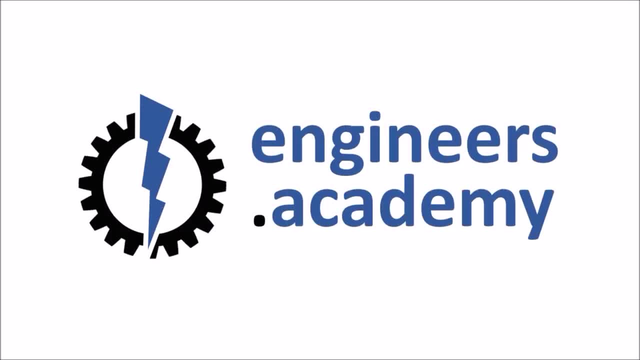 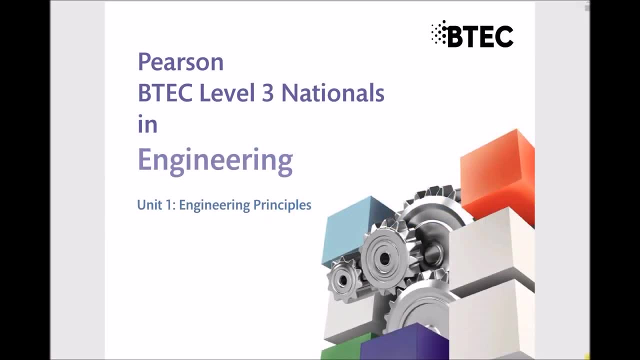 Hello, this is Andy from the Engineers Academy, and in this video series we're going to be looking at work solutions to the Unit 1 Engineering Principles exam, which will be sat by students studying BTEC Level 3 Nationals in Engineering. Now the document that we're going to be referring: 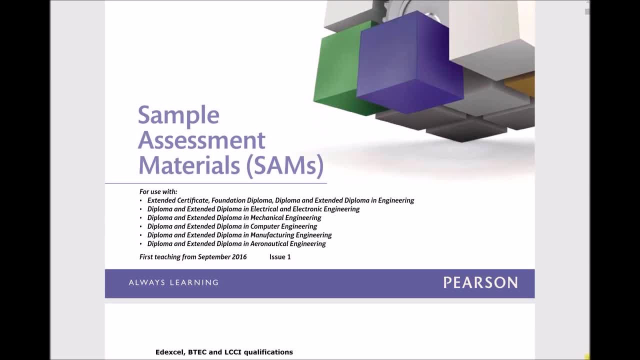 to today are the sample assessment materials that are, or have previously been provided on the Edexcel website, and the document that we're going to be referring to in particular is Issue 1 of the sample assessment materials. Question 9 reads: when designing a bridge, it's important. 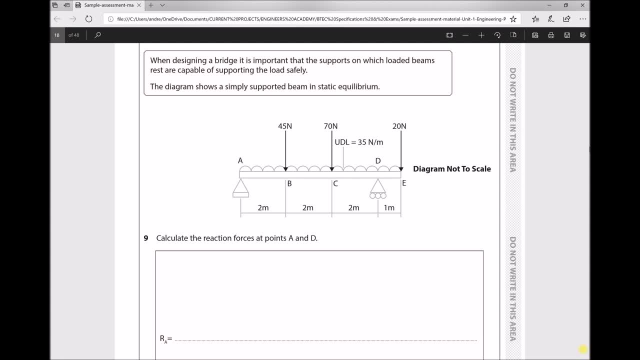 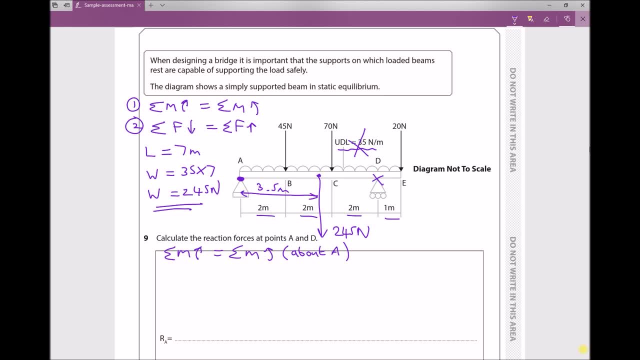 of those forces and if we imagine the beam pivoting at point a, we can see that the 45 newton force is causing the beam to turn clockwise, the 70 newton force is causing it to turn clockwise, the 20 newton force is causing it to turn clockwise, and so is the weight of 245 newtons. 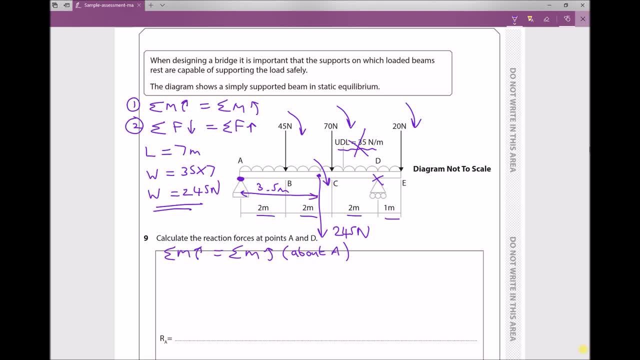 and in fact the only force that's trying to turn it anti-clockwise is our force at point d, the reaction force at point d, so some of the clockwise moments, and a moment is a force times a distance. so we have 45 newtons and the 45 newton force is 2 meters from the pivot. 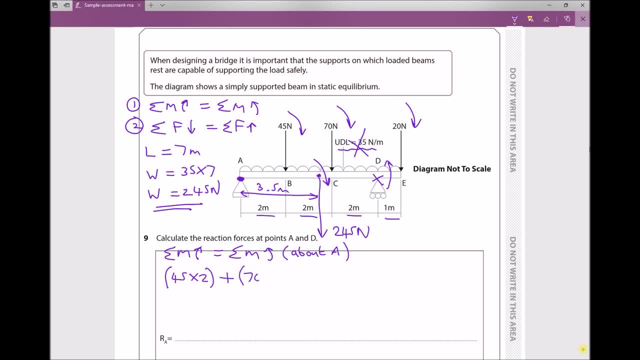 to that we're going to add the 70 newton force, and the 70 newton force is 4 meters from the pivot- just remember to take the distance back to the pivot each time- and then we have a 20 newton force, and that's distance is 7 meters from the pivot. 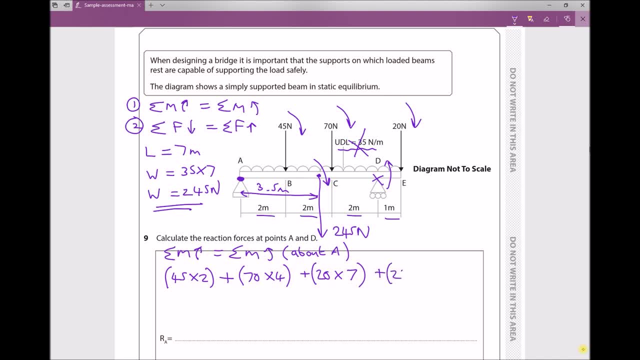 and not to forget the weight, which is 245 newtons at a distance of 3.5 meters from the pivot. now all of that is going to equal our reaction at d, so r subscript d times its distance from the pivot, and we can see from the diagram there that that's. 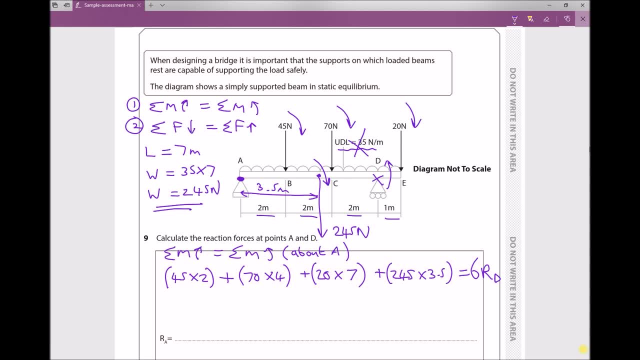 6 meters from the pivot. so 6 rd is the same as 6 times rd. so my next step is to simplify the left hand side, and all i'm going to do is multiply that out. so 45 times 2 plus 70 times 4 plus 20 times 7 plus 245 times 3.5 equals 1367. 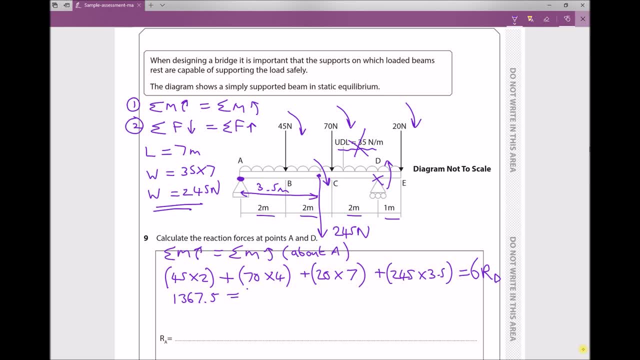 0.4, And that still equals 6 rd, because we haven't done anything to our right hand side. well, what we have here is a simple linear equation. if we want to get rd on its own, all we need to do is divide each side by 6.. 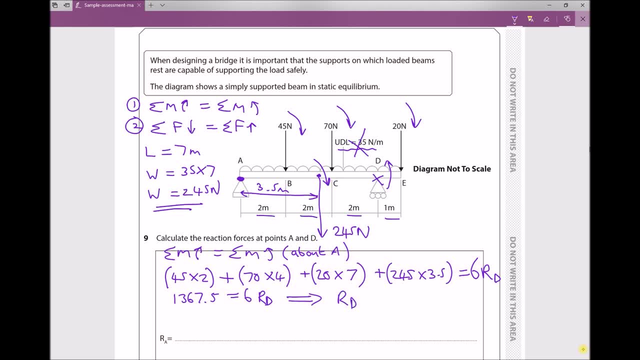 so what we're going to end up with is that the reaction at d equals the 1367.5 over 6, which gives us 227.9may di diminish 0.317, because we yet to multiply each surface over this equation evolving. to see what happens now. this will be equal to the energetic part here, rd over 6, not the velocity. but 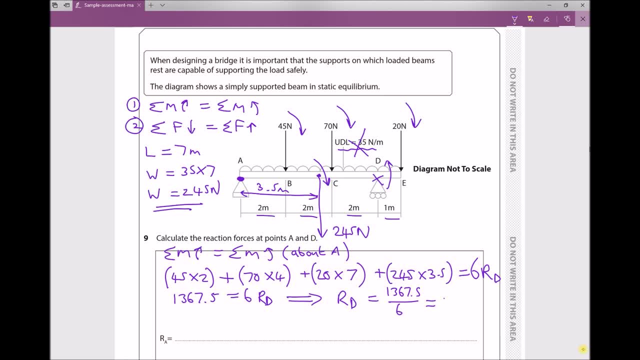 what we do want to do in the 핀 replied: theomorph, and then we'll divide it by six, so that we're going to start the study and we're going to. Mommy says the corner values tend to be pronouncedije 9, we'll just go to one decimal place: 227.9 Newtons. 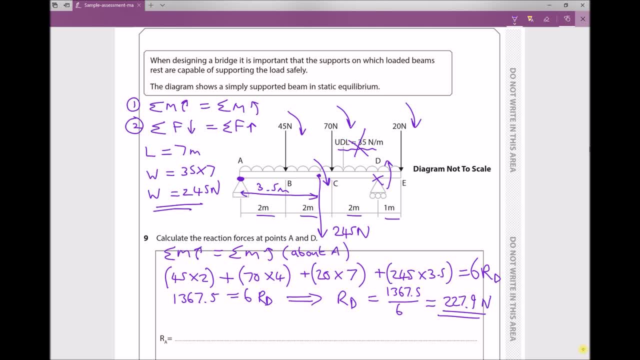 Now we just need to take a little bit of care here, because if we look what the final answer is asking for here, it's actually asking for RA. So we'll come back and we'll fill RA in in a moment. Now our second condition for static equilibrium states the following And: 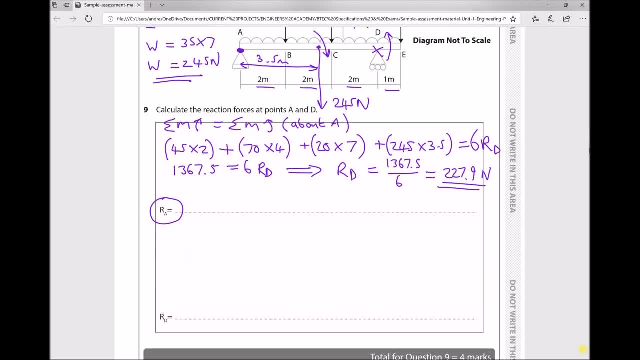 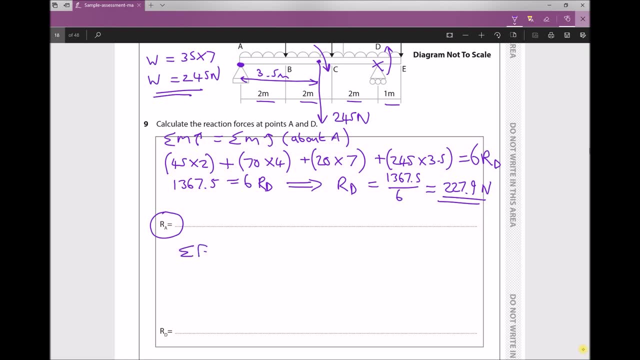 we'll move into the next bit of the working area. The second condition for static equilibrium states that the sum of the forces pushing downwards equals the sum of the forces pushing upwards. Now we're only dealing with forces here, not with turning moments. So if we refer, 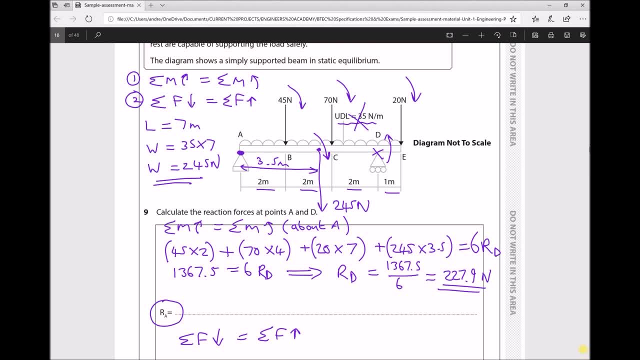 back to our diagram. we can see that the following forces are acting downwards: We have 45 Newtons acting downwards. We have 45 Newtons acting downwards. We have 45 Newtons acting downwards. We have 70 Newtons acting downwards. We have 20 Newtons acting downwards. But we also have: